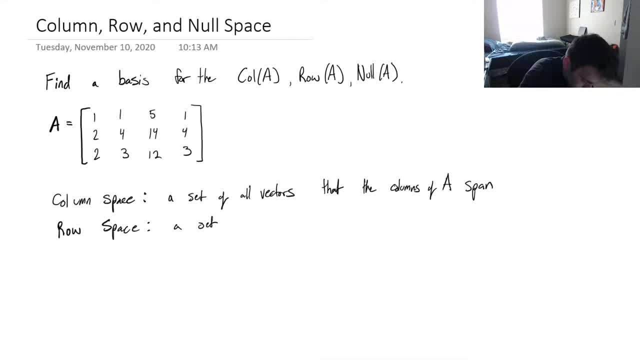 It's also a subset, so a set of all vectors that the rows of A span Right. So, similarly, if we were to take these rows, These rows, if we took all possible linear combinations of- and typically we take the transpose of those rows so we read them vertically right. 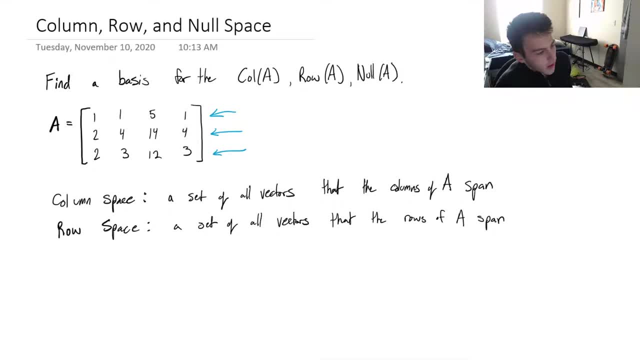 So we would have three vectors in R4.. It's just the span of those rows of those vectors, right? So what is the null space? Well, the null space is just the set of all vectors which are solutions to Ax equals the zero vector. 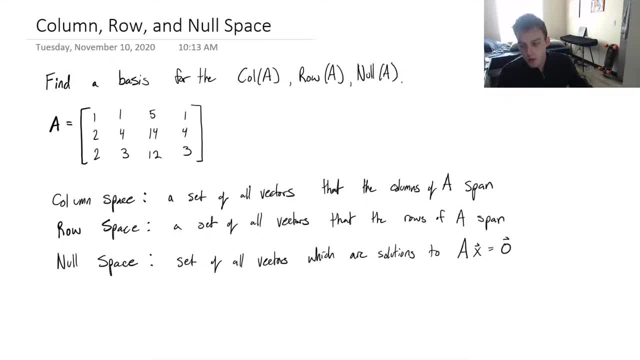 So how do we actually compute these things Right? Okay, And let me be extra clear here. actually, The set of all vectors which are solutions to Ax equals zero. Remember, solutions means vectors X that we can plug in to this. that'll be multiplied by our matrix A and it'll be equal to the zero vector. 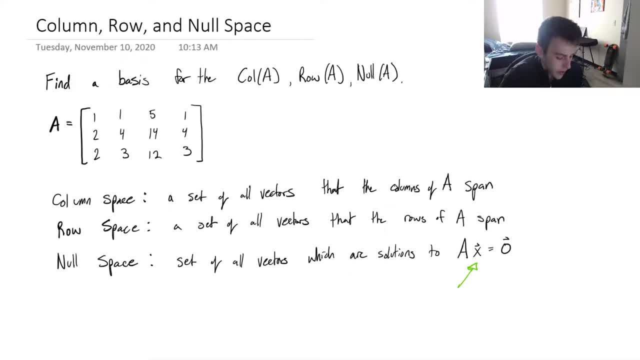 So, as you learn more about linear combinations, you can think of it as taking that vector X, applying A, which is just this linear transformation where we shift space and what are. it's the set of all vectors that if we shifted space by applying linear transformation A. 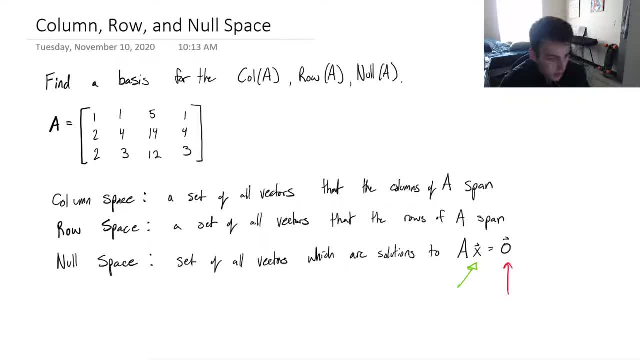 they will land on this zero vector right there or it'll land at the origin. So what vectors can we plug into that matrix vector product that it will be equal to the zero vector? So how do we compute these things? Okay, 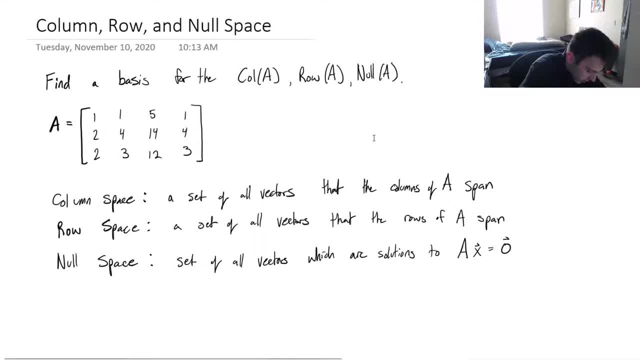 Well, if we actually just row reduce A, then it'll tell us quite a few things, right, And depending on the way that we interpret the result of our reduced row echelon form. So let me row reduce this right now and I will get back to you in just a sec. 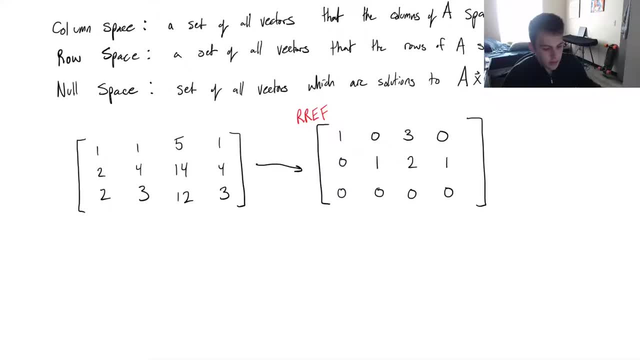 So this is the reduced row echelon form. I skipped it for sake of time in this video, But I just want you to remember that we're dealing with a homogenous system, which means that this augmented side, we don't really write it, but it's going to be 0, 0, 0, right. 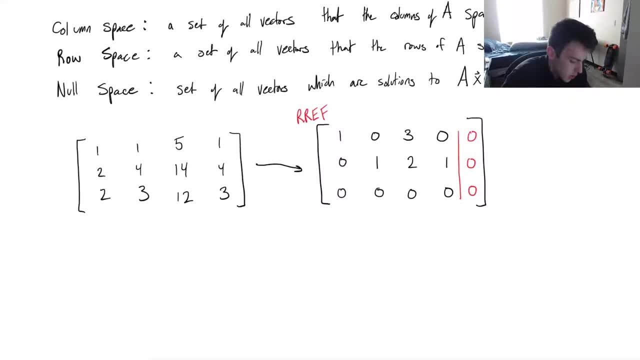 That's not affected by row operations, so we don't write it, But just a reminder that we've got equal 0 in all of these separate equations here. So if we were to consider this for the null space, then we want solutions to all of these X values. 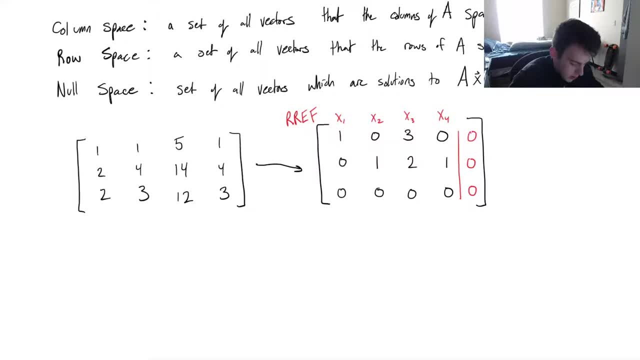 that we get that we're equal to the 0 vector. So it's like: here we have three separate scalar equations for some, but with four variables, X, these being the coordinates of our X vector, And we're solve. we just want to solve this matrix. 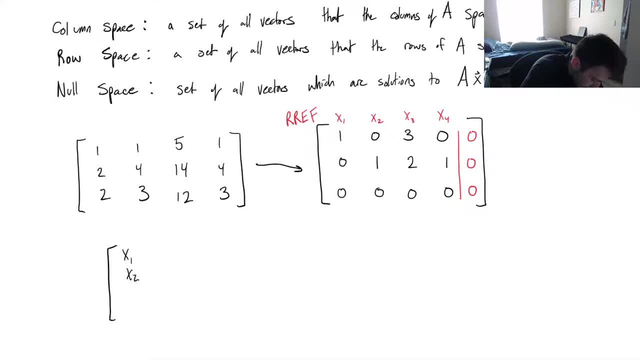 So here we've got X1, X2, X3, X4.. And well, we know here that X3 and X4, these will both be free variables, since there's no leading entries in this column. 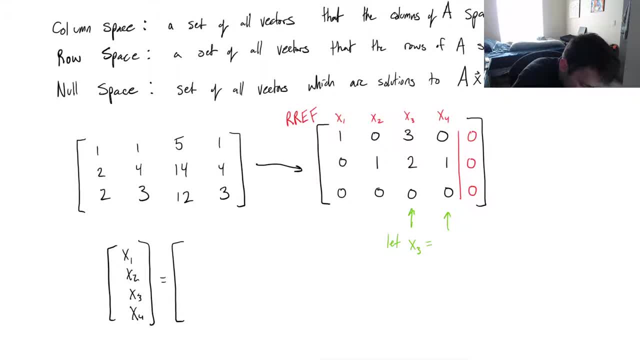 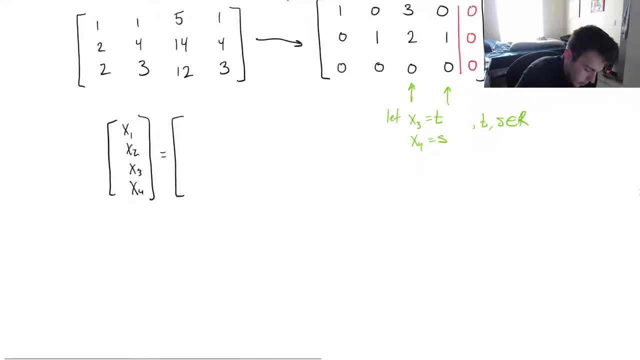 So let's let X3 be equal to T and let's let X4 be equal to S, where T and S are real numbers. Let me scroll down a little. So X1, reading our solutions off of this- X1 would be minus 3T. 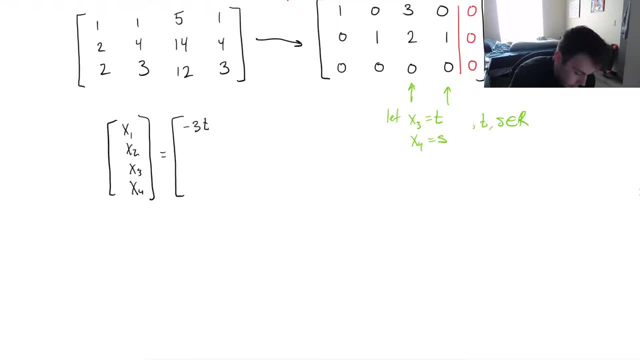 X2 is going to be minus 2T, minus S. and then X3, we said was T, X4, we said was S. Great, So this right here, any values of T and S will be solutions to Ax equals 0, right. 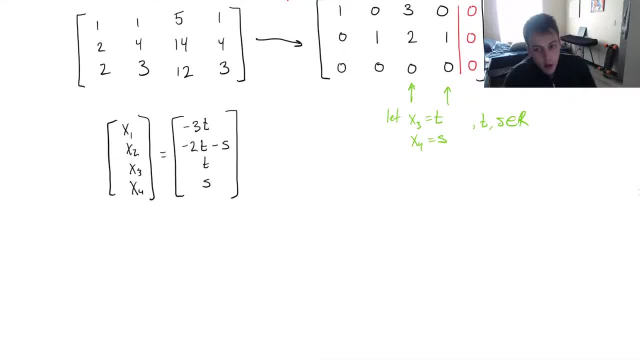 So we need to get this in the form of the like a set of all vectors, Right? So what can we do here? Let's just break this up. Let's have T multiplied by a vector minus 3,, minus 2, 1, 0,. 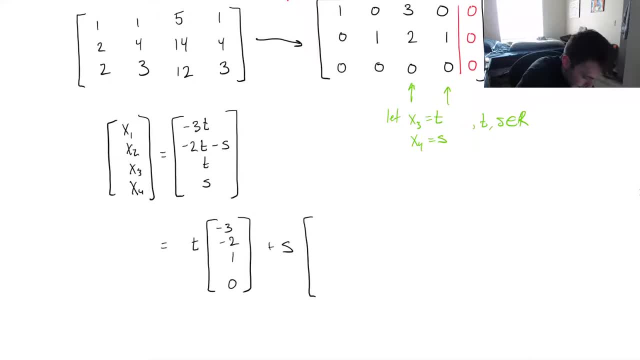 plus another scalar times, another vector. This we got 0, negative: 1, 0, 1.. Right, This is the exact same thing. We just broke it up And you see how we broke this up and you can see here: 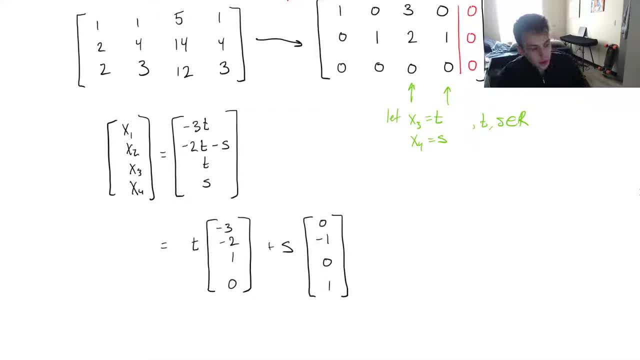 that this is very similar to like the form of like linear combination: Instead of a C1 and a C2, we have a T and an S, But they're both constants, so it means the same thing. So what this is telling us here is that 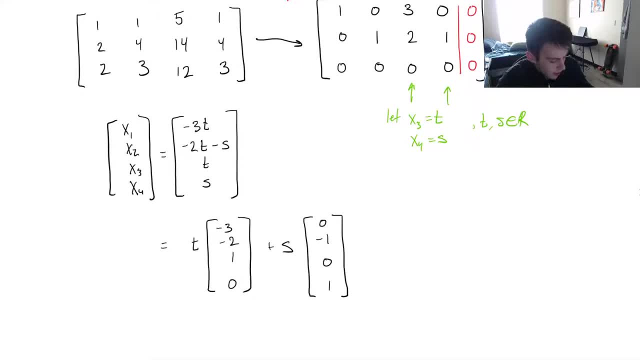 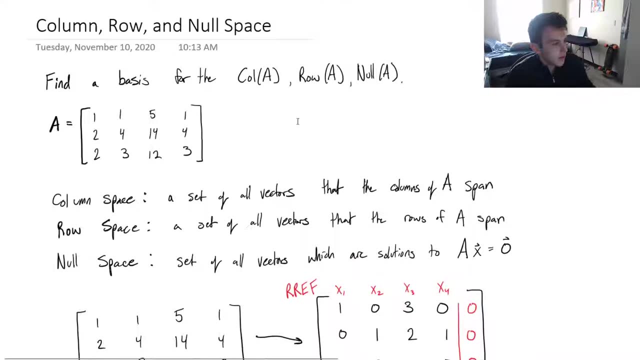 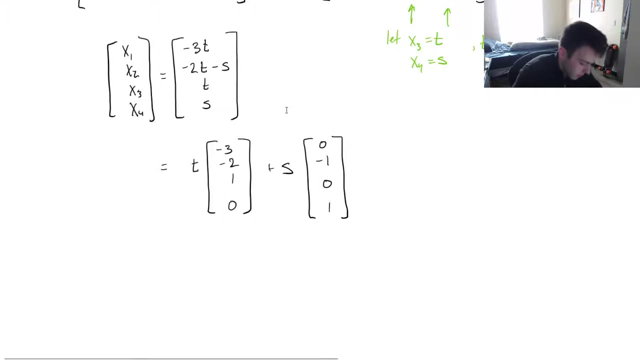 this is just the span of these two vectors, Right? And the question's actually asking us typically like we're finding the basis for these column row and null space, right? So if we're finding the basis, then we are looking for a linearly independent set of vectors. 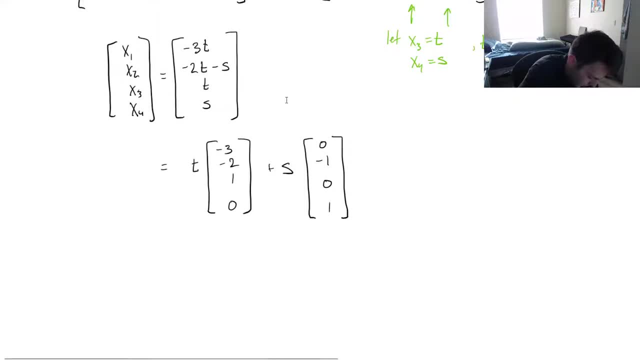 that spans the entire vector space, right, And we know right here that this here we can just rewrite this as the span of these two vectors, because this is what it is Right. T and S are just scalars, so this is just the linear combinations. 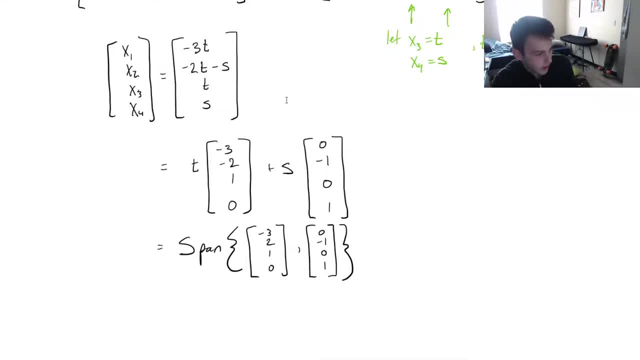 That is just all of these, The linear combinations of those two vectors. So this right here, like this, is our null space, Right? So if we're looking for the basis, it just needs to be a linearly independent set of vectors. 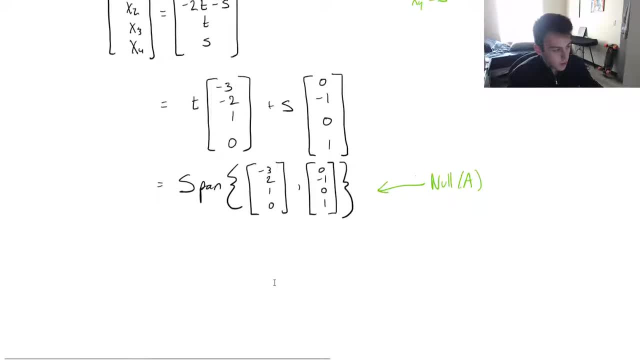 that span the entire null space. So clearly, like by definition, we can tell that these two vectors span the entire null space And they're linearly independent. We don't have to prove this because, since there's only two vectors here, 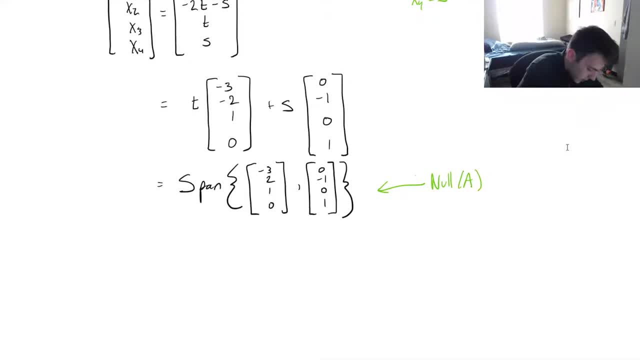 we can tell that they're not scalar multiples of each other. But if you had more, you should prove that they're linearly independent before stating it's a basis. So now we can say that. we'll say, therefore, the basis for the null space of A. 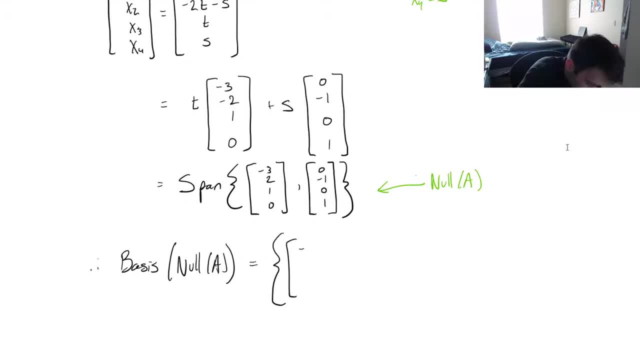 is equal to. and it's just these two vectors. Oh, and I missed a negative, My bad. Okay, great. So null space done out of the way. Let's take a look at the column space now. So remember. 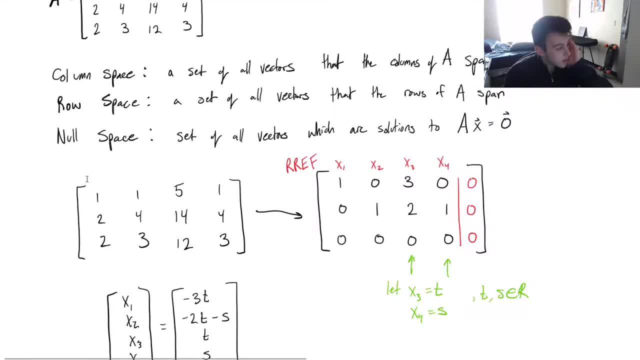 the column space is the set of all vectors that the columns of A span. So if we look here, let's consider this like a linear combination of vectors. We'd set up the system the same way, So instead of having these as our x1,, x2, and x3, and x4,. 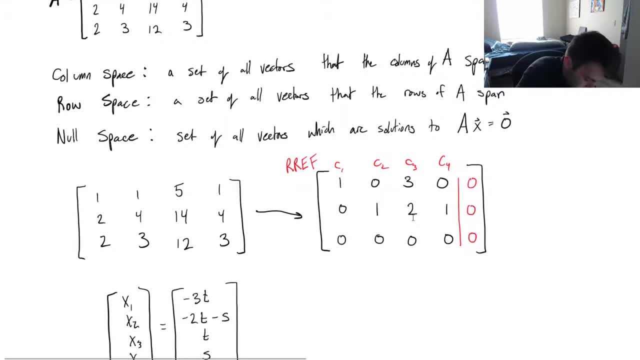 this will be c1, c2, c3, c4.. Think of it like c1 times 122 plus c2 times 143, plus c3 times 5, 14, and 12 plus c4 times 143 equals the zero vector right. 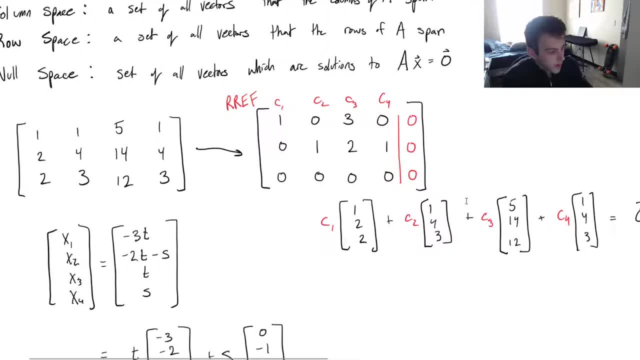 We set up the same system of equations to solve this right. So we can tell here that since c3 and c4 are free variables- right, because they don't have leading entries in these columns- that means that we have solutions to what we just wrote out. 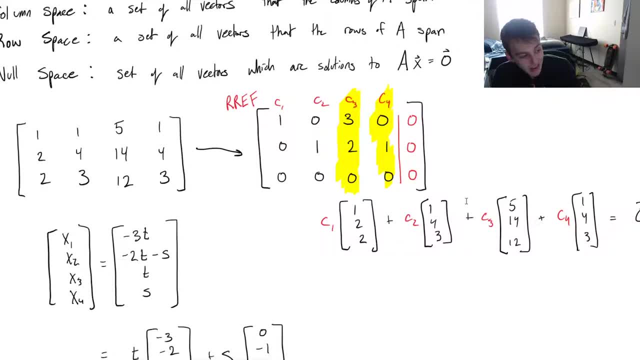 when c3 and c4 are not equal to zero, because they can be anything. So that's making these set of vectors linearly dependent. right, These four vectors here. But if we were to remove c3 and c4, then we would have linearly independent vectors. 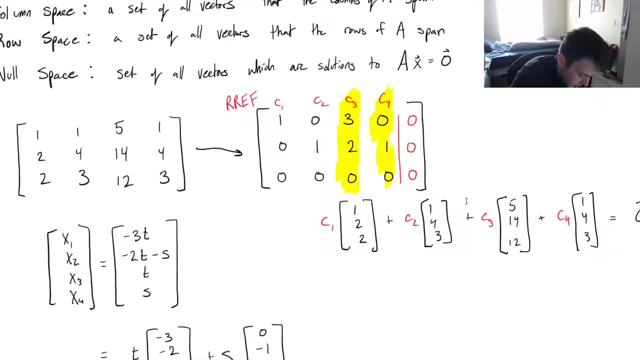 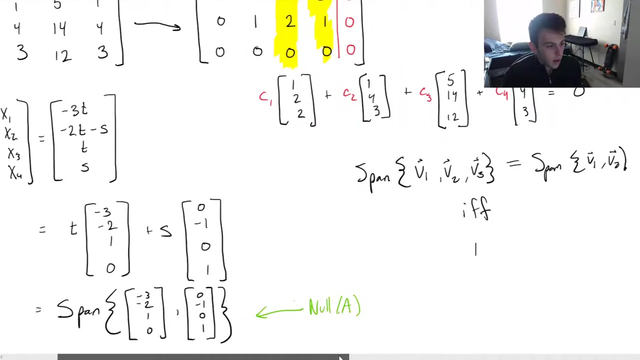 in our set right. So because, remember the span, like there's a theorem we know: the span of v1, v2, v3 is equal to the span of just v1 and v2, if, and only if, v3. 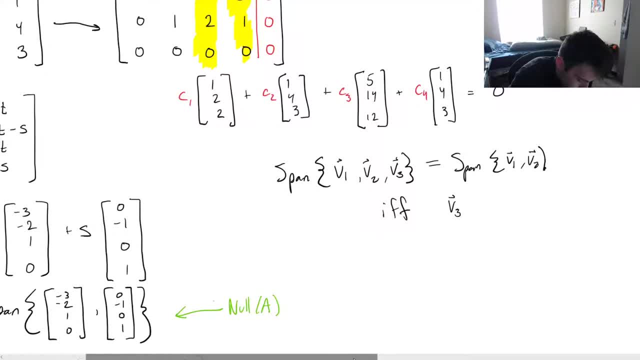 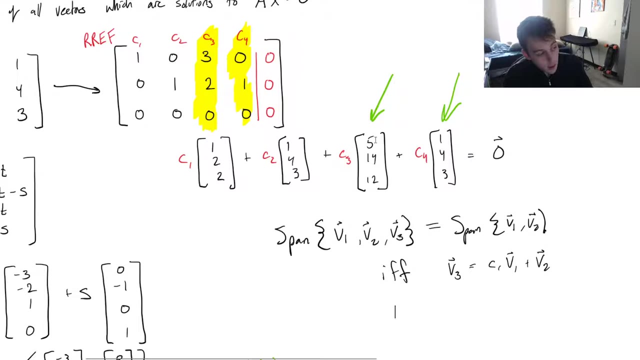 is a linear combination of the other vectors in the set right. So we know that v3 and v4, in our case right, this one and this one. we know that, since there's solutions when c3 and c4 are not equal to zero, 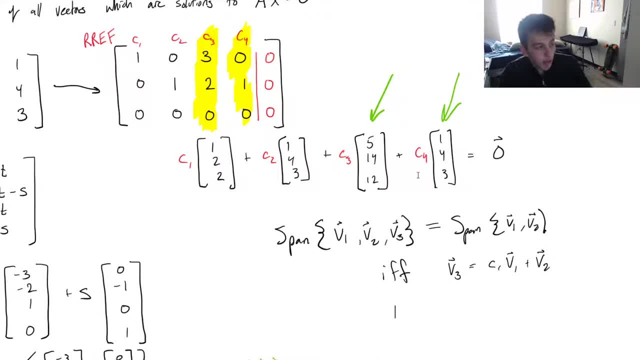 we know that those can be expressed as combinations of the other vectors in the set. So what we do is we remove those and we can just express the span of the columns in its simplest form, removing out all of the unnecessary vectors from our span. 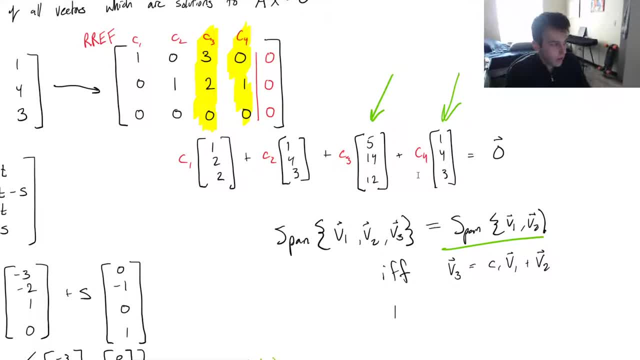 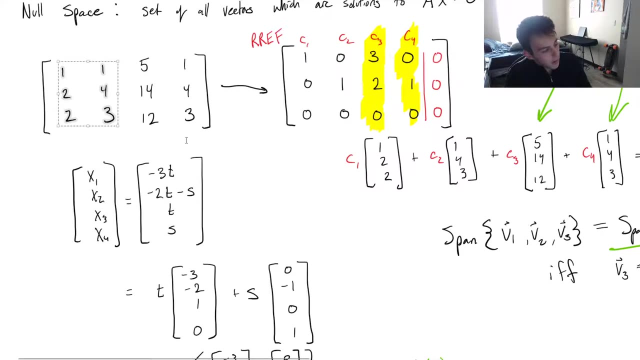 essentially getting it into like this form over here. So we take: we see that c1 and c2 are those linearly dependent vectors or independent vectors, sorry, So we'll take a look at those vectors here right from our a form. 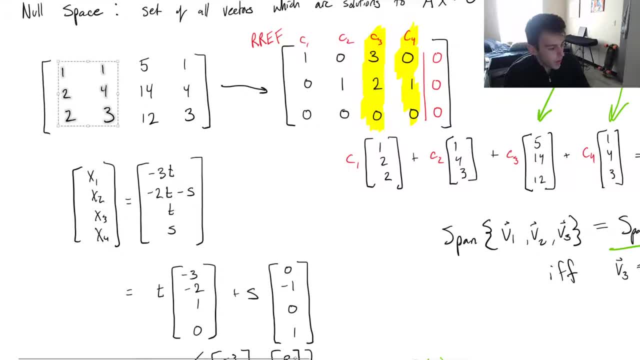 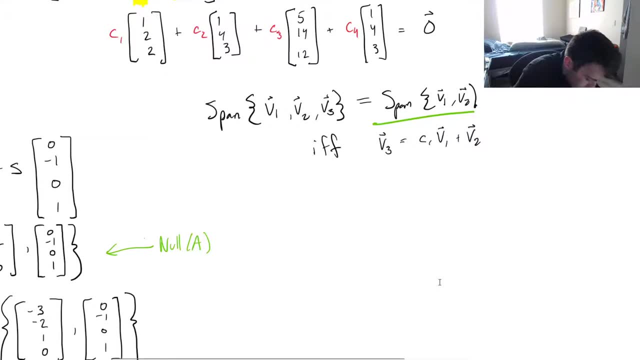 of the matrix 1, 2, 2 and 1, 4, 3.. So from this we can say that the oops, the column space, is equal to the span of those vectors 1, 2, 2 and 1, 4, 3.. 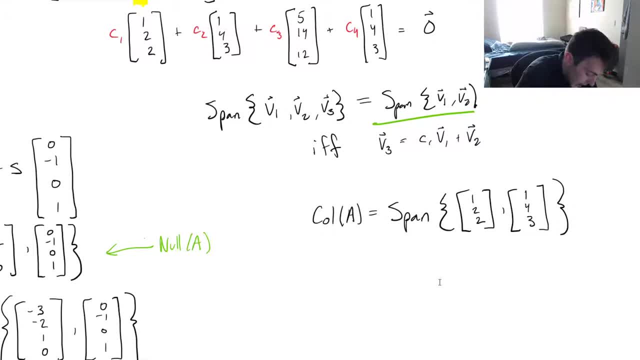 Right. So the basis, very similar to the to the last one, is just a set of linearly independent vectors which span the entire column space. So clearly, like by the definition of the column space, the two vectors in our span. 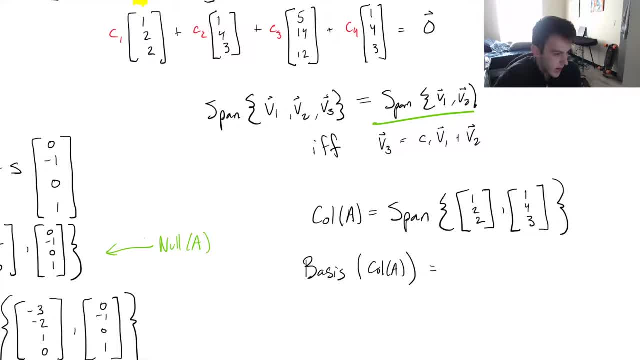 will span the entire column space And they're linearly independent. we can tell They're not scalar multiples of each other. So, and remember, that's only the case because we have two vectors here. If we had more we should check. 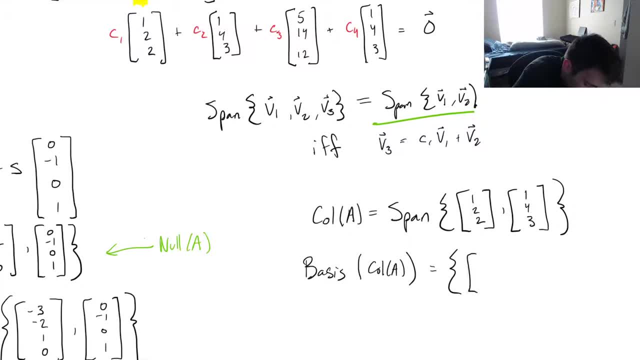 So the basis, the basis would be 1, 2, 2 and 1, 4, 3.. And I just want you to keep in mind the dimension of the column space, or AKA, the number of vectors in the basis. 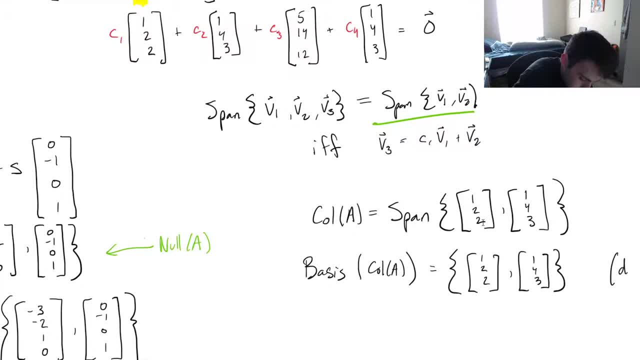 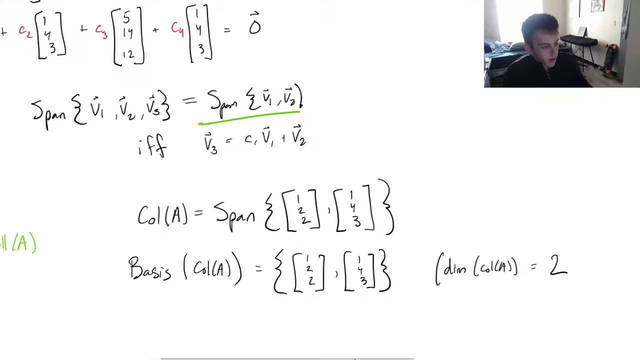 for the column space is 2.. Just keep that in mind. Equals 2.. Okay, And finally, there's one more thing that we, that we're asked to find, And it wants us to find: the basis for the row space. 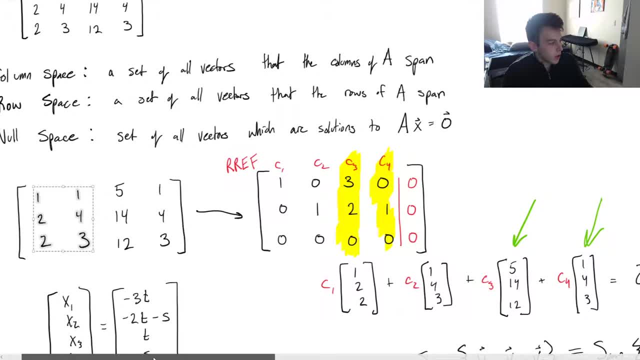 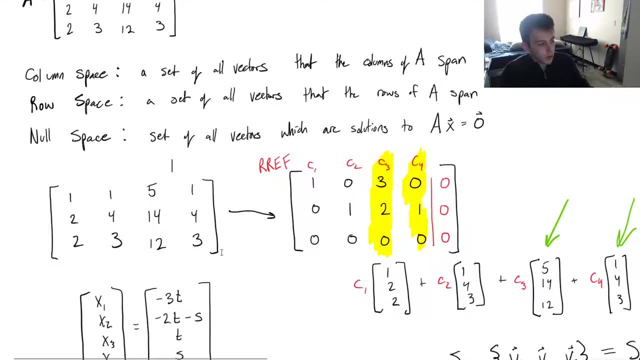 And the row space is very similar to the column space. It's the set of all vectors that the rows of A span, Right. So instead of the, the columns. like what's the simplest form of the span of the columns? what's like the simplest form. 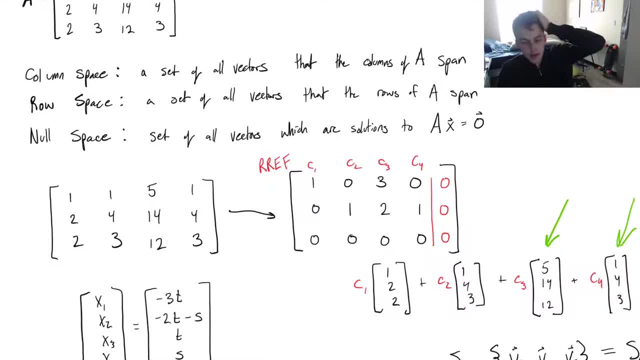 that we can span the rows And, similarly, we just want to take a look at, like, what's the simplest form that we can express the span of the rows, And there's a theorem that tells us that the reduced row, echelon, or the span of the rows, 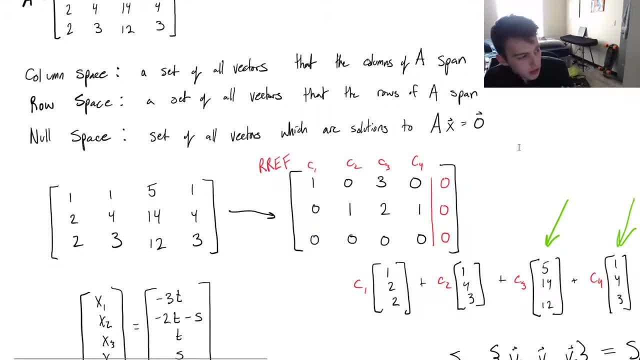 of the reduced row echelon form is going to be equal to the span of the rows of the just the A form before we apply any elementary row operations. So it doesn't matter which one that we look at And we can clearly tell here. 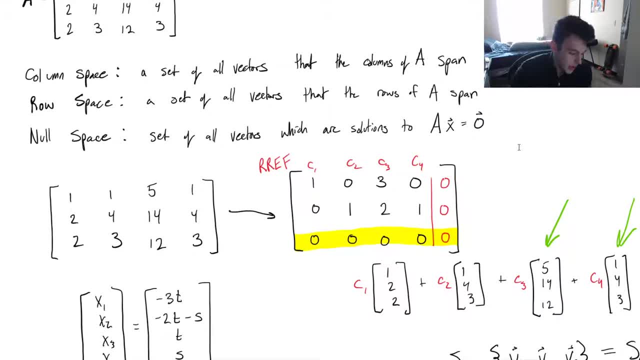 that, like this row of zeros, is not going to add anything to our span. So what we? just what we do is we take these two vectors here, these two rows as our non-zero rows of the reduced row echelon form, And those two vectors. 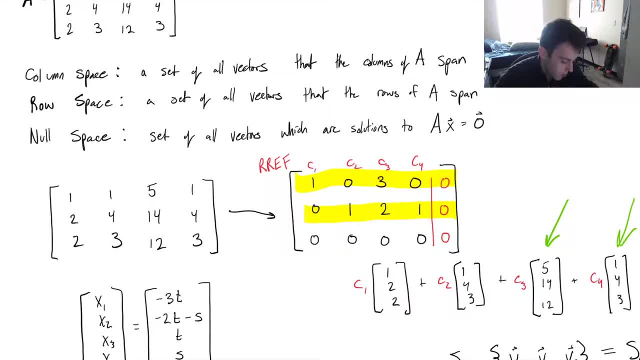 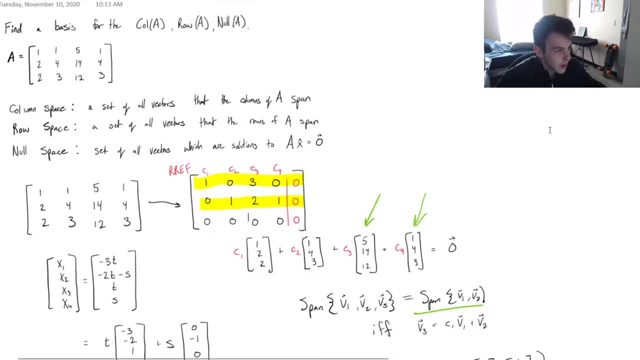 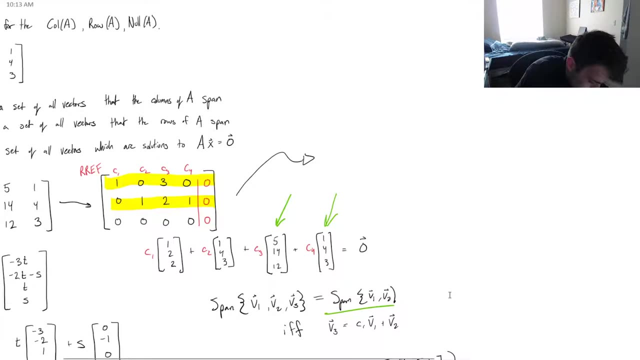 are going to be our row space, So let me zoom out a little bit here. I guess I'll write it up over here. So the row space of A would just be the span of one zero, three zero and zero one, two, one. 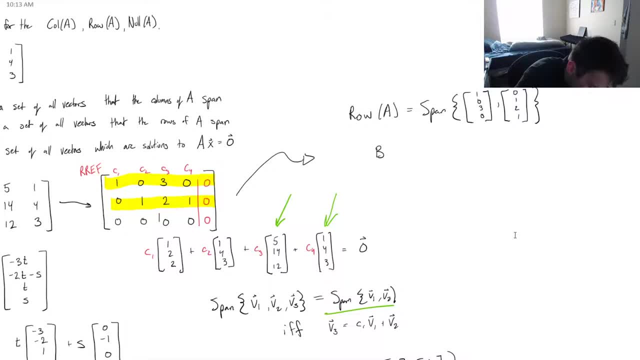 Right And very similar to the last examples. the basis of the row space of A, what we know, it's got to be a linearly independent set of vectors and it should span the entire row space. So clearly these two vectors. 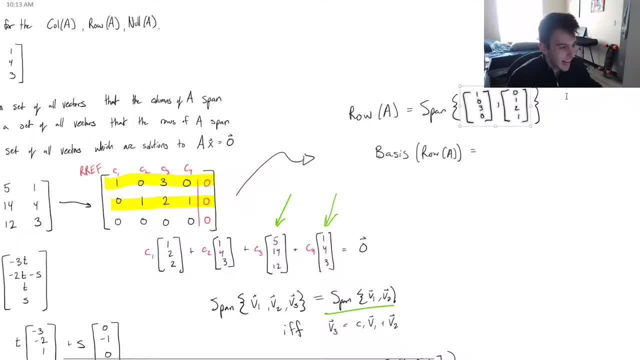 would span the entire row space, like by definition, And then they're linearly independent, since there's only two vectors. They're non-zero, they're non-parallel, So those two vectors will be linearly independent. So our basis will be. 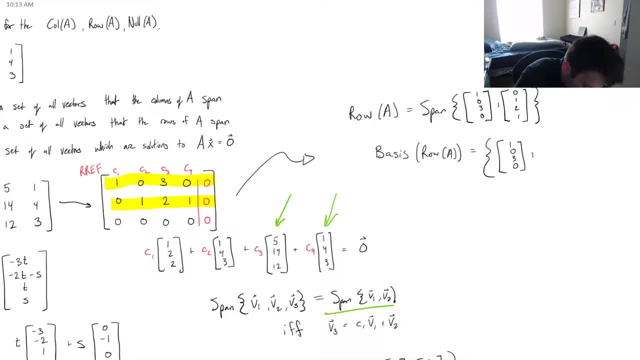 one zero, three zero and zero one, two, one. Great. So this would be our basis for the row space. And another thing I just want to draw your attention to. you'll see here that the dimension of the row space of A 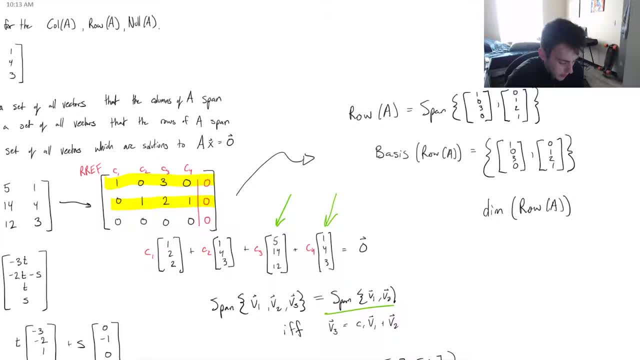 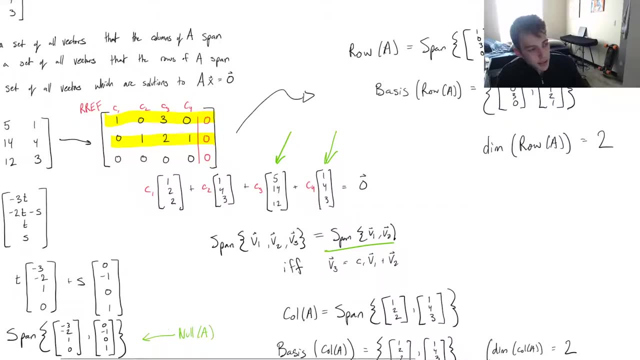 or the number of vectors in the basis for the row space of A is also equal to two. So something that you might want to keep in mind is that the dimension of the row space of A is equal to the dimension of the column space of A. 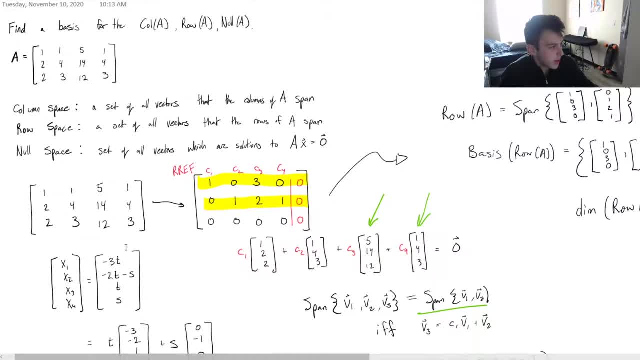 So let's just go over everything and make sure that we understand it. So: column space: set of all vectors that the columns of A span, Row space. similarly, it's the set of all vectors that the rows of A span. 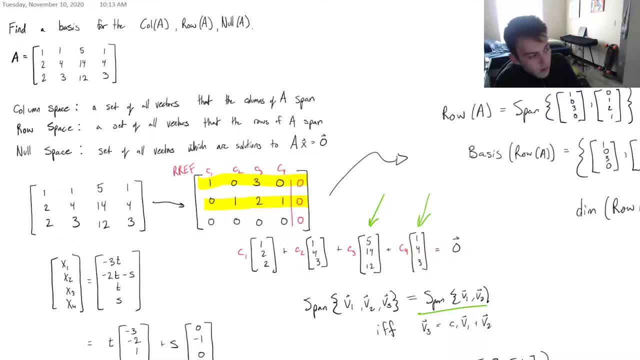 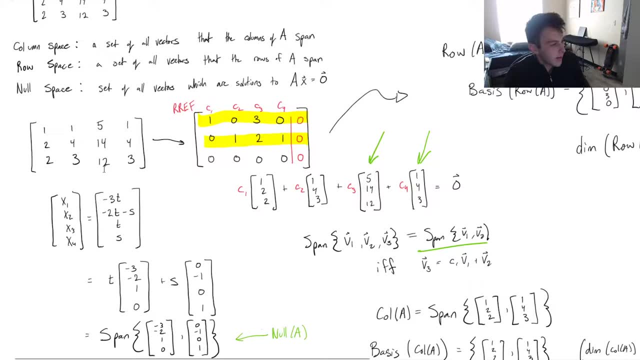 So the null space is just going to be the set of all vectors which are solutions to. Ax equals zero. So when we were calculating that, all we did was take the. we described the solution to our homogenous system, we broke it up. 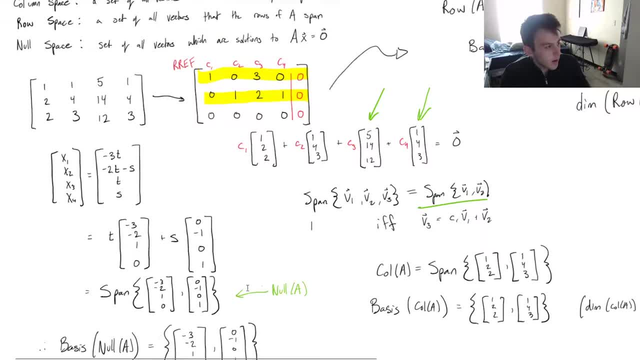 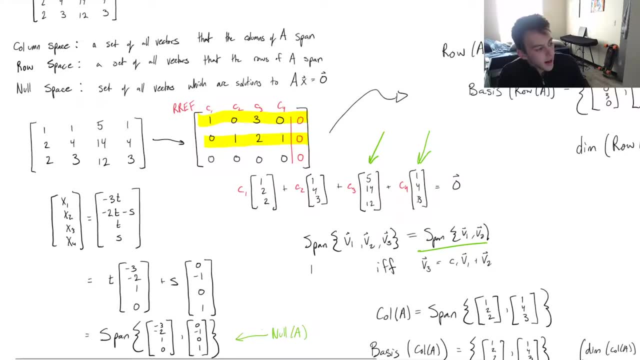 and we took those two vectors as our basis For the column space. we row, reduced the linear combination of those columns and then we removed all of those vectors that can be expressed as linear combinations of the other ones in the set And we just yeah. 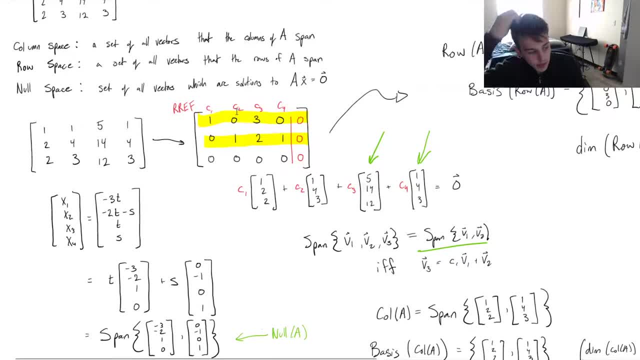 so we took those, the linearly independent columns, as our basis for the column space of A And the row space of A. all we had to do was take a look at the reduced row echelon form, take all of the non-zero rows of that matrix. 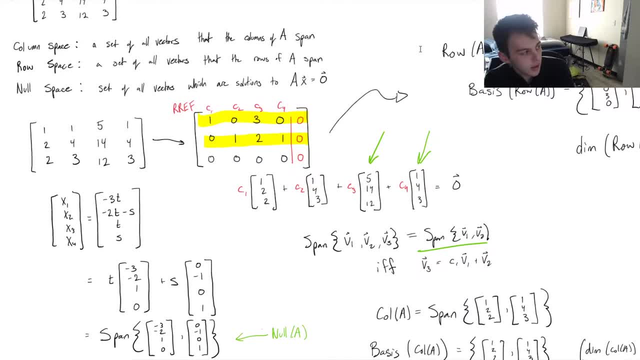 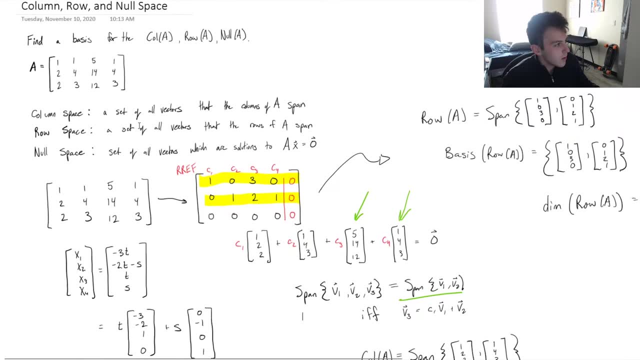 since it's the same as the row space of the before we apply any elementary row operations to it. So I hope this video was helpful And if you have any more questions, feel free to drop a comment and I'd be happy to respond.